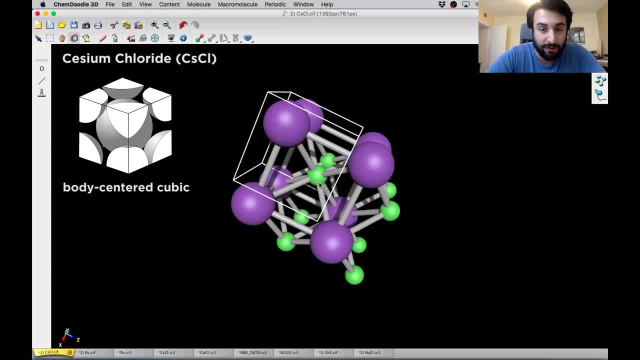 before. but there's an additional atom in the center of that lattice, And so if they were all the same element, we'd be calling it a body-centered cubic structure, And a lot of metals do crystallize that way. But because of that we're going to be calling it a body-centered cubic structure, And so 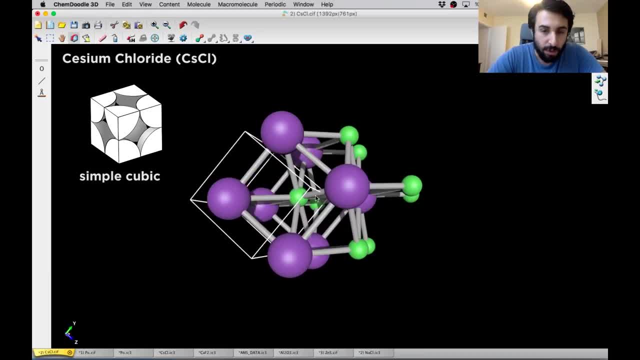 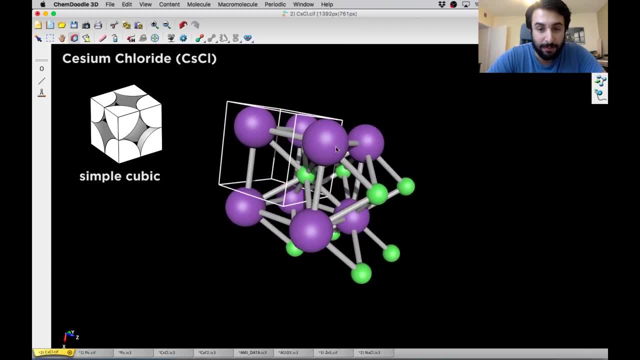 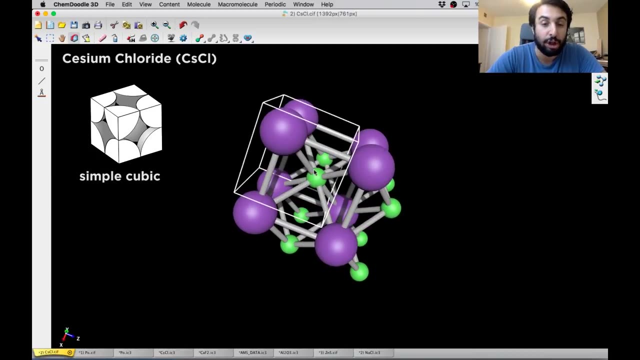 because this is an ionic compound and we have two different elements. we are not going to call it a body-centered cubic. It is actually still a simple cubic structure. if we consider the cesium ions forming a simple cubic structure, And then the chloride ions are filling all of the cubic holes. 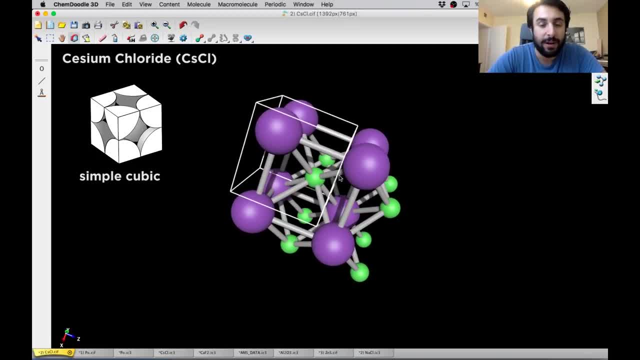 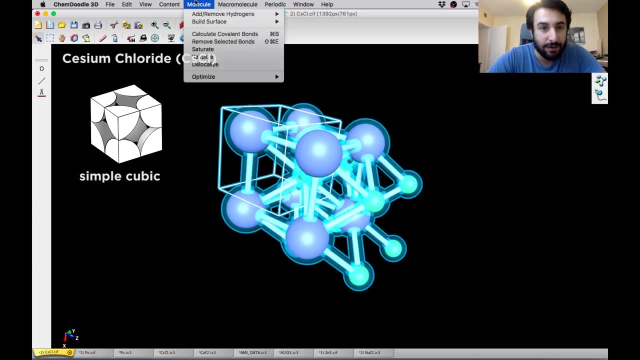 So, when ionic compounds crystallize, they want to make the best use of the space as possible. They want to make the best use of the space as possible. They want to make the best use of the space as possible, And so that's what this is going to form, And we can even take a look at this without 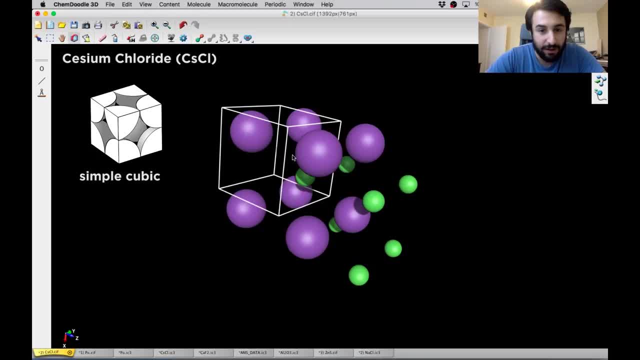 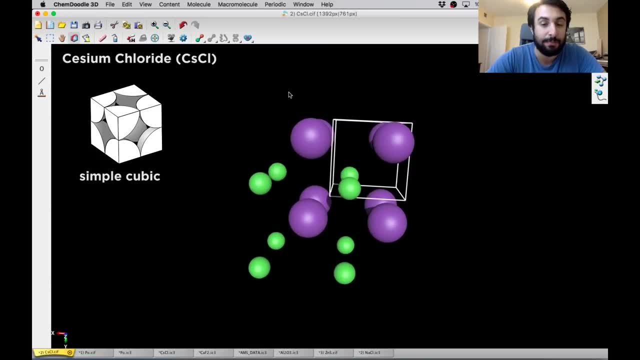 those bonds, if we want to see this a little more clearly. So here we can see that this is a simple cubic structure And the interesting thing is, you can consider it a simple cubic structure with either of the elements. So we could consider the cesium ions as forming the simple cubic structure. 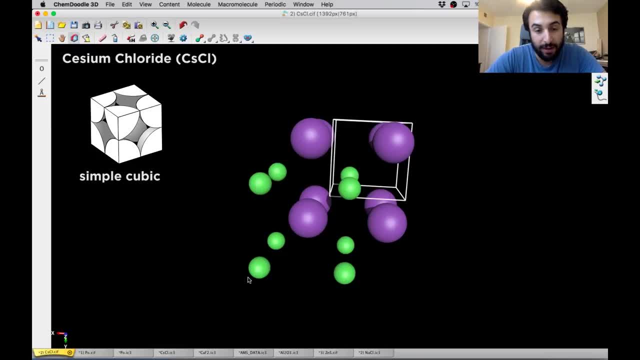 and the chloride ions occupying the cubic holes. Or we could flip it and we could say that the chloride ions are forming a simple cubic structure and the cesium ions are filling the cubic holes. Either way, whichever way you want to look at it, it's the same thing, And let's build. 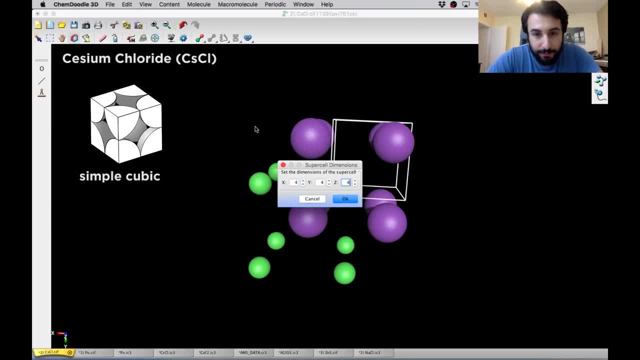 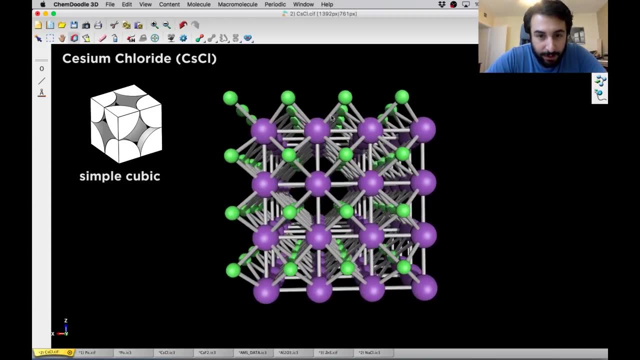 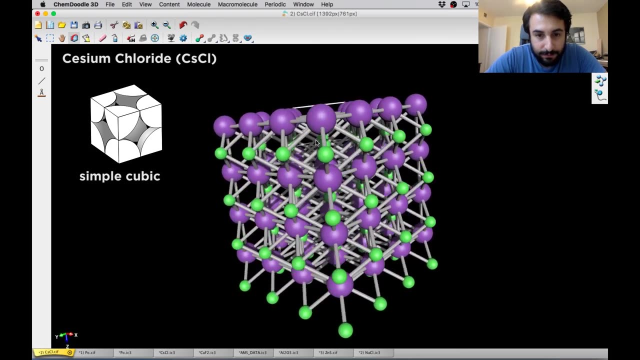 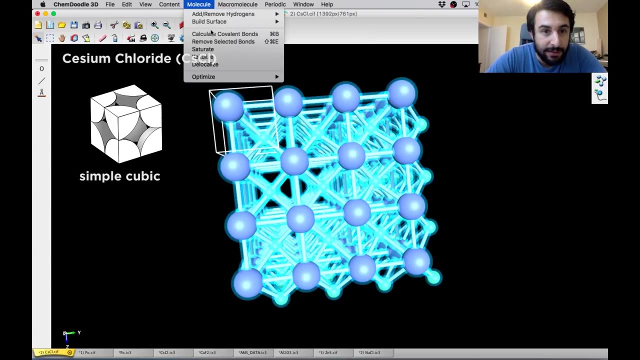 this out a little more. How about let's do four, And now we can really see quite a bit of structure here. We can rotate this a number of ways, And that's what we're looking at Once again. let's go ahead and remove those bonds. 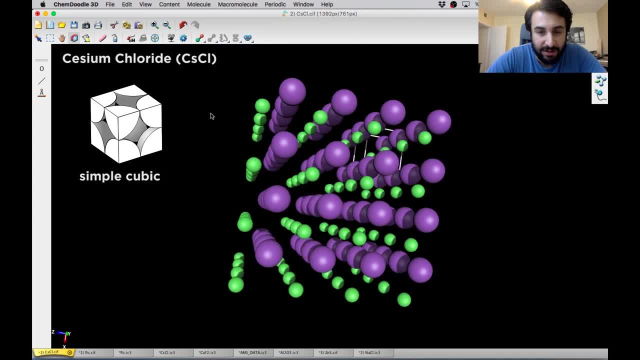 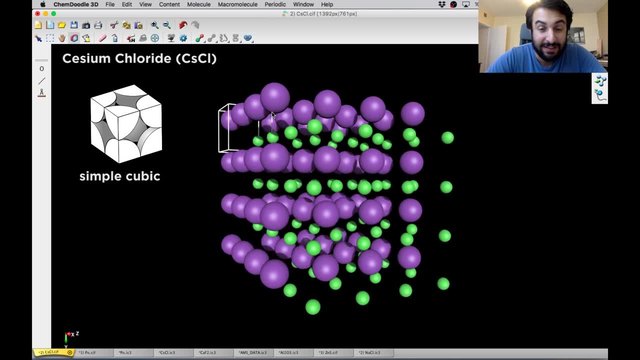 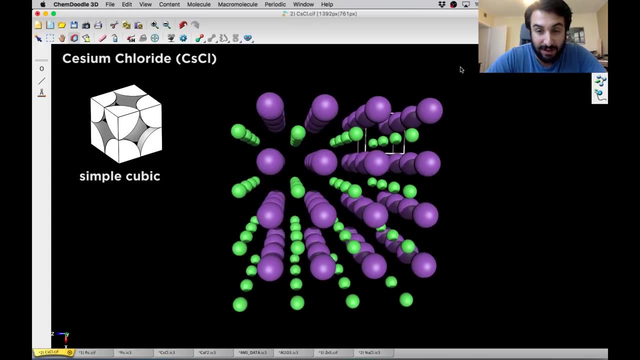 And we can really see this is still quite a simple structure, right? This is about as simple as ionic compounds can get, And of course this depends greatly on the relative sizes of the ions. here The sizes of the ions are quite similar, But this changes a little bit when the sizes of 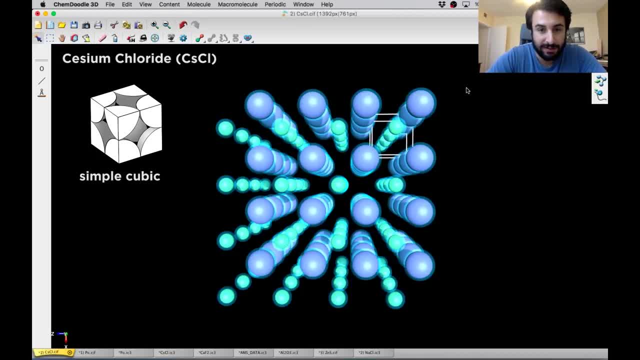 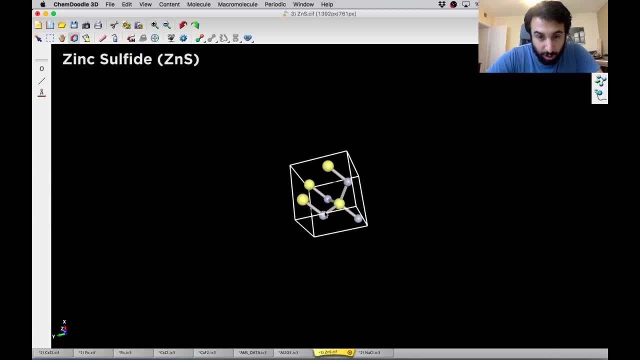 the ions become quite different. So we can see here that the sizes of the ions are quite similar. So let's take a look at another one. Let's get rid of this. Okay, we're now looking at zinc sulfide. So the zinc ions are here in gray. 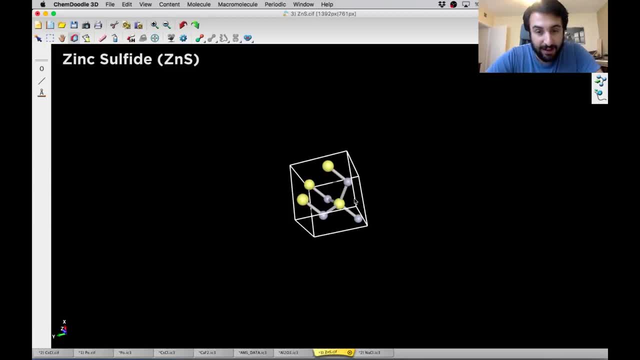 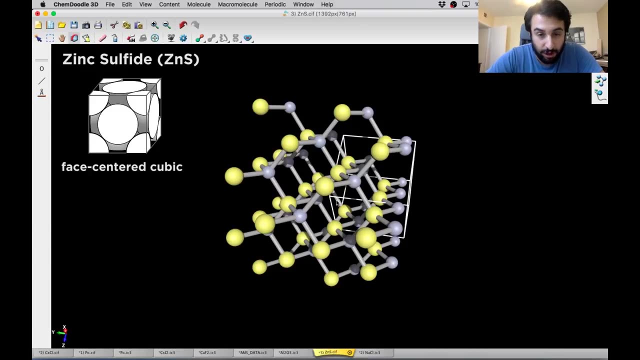 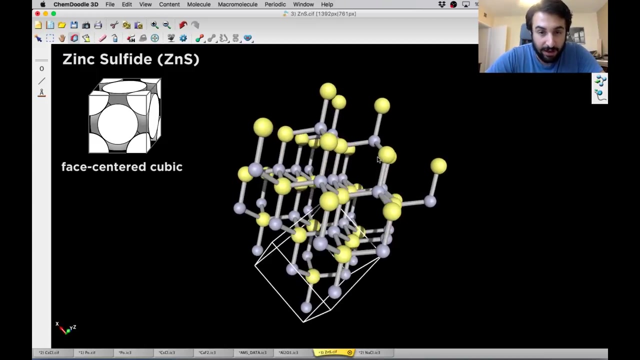 and the sulfide ions are in yellow, And so let's build this out just a little bit so we can get a better sense of this unit cell. And this is actually a face-centered cubic structure. So that is where the sulfide ions are forming, the unit cell, centered in the faces of the cube, And then the 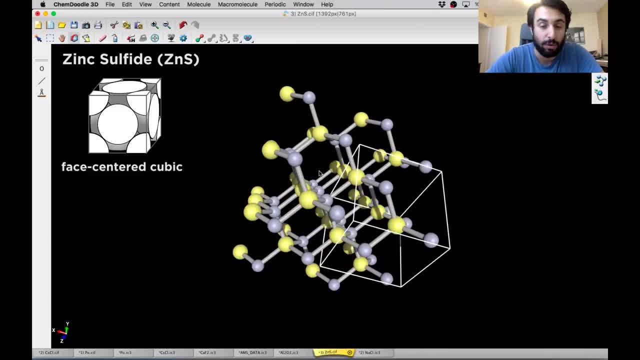 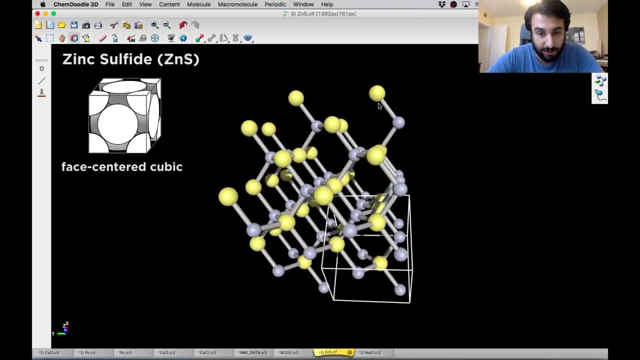 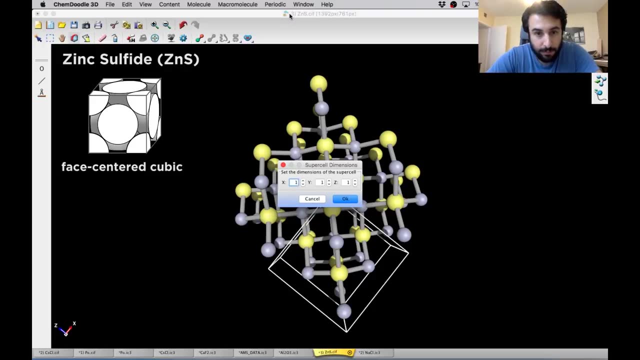 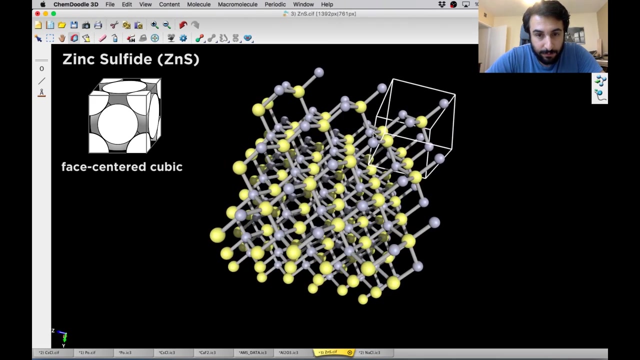 zinc ions are filling the tetrahedral holes formed by that structure. So this is what this one looks like, And we can build that out even a little more. Let's just do three, And so we can see that this is a little bit of a different structure, And this is mainly because 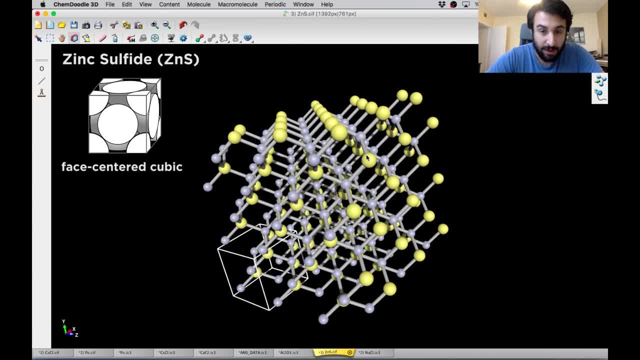 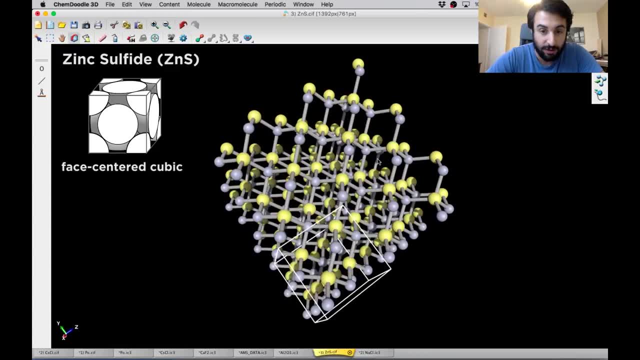 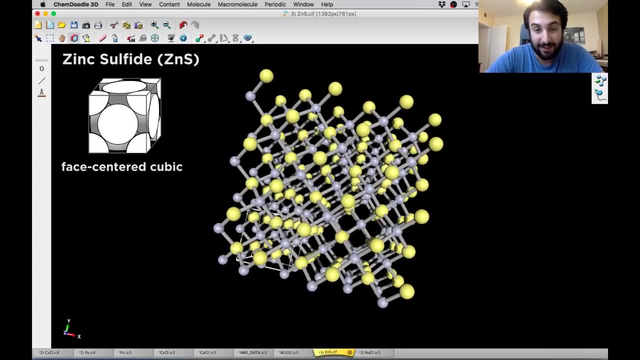 of the discrepancy in the sizes of the ions. So the larger chloride ions are going to form that lattice, And then the zinc ions are going to just fill in the gaps. They're going to fill in those tetrahedral holes, And so this is typically the case, that the anion is going to form the unit cell. 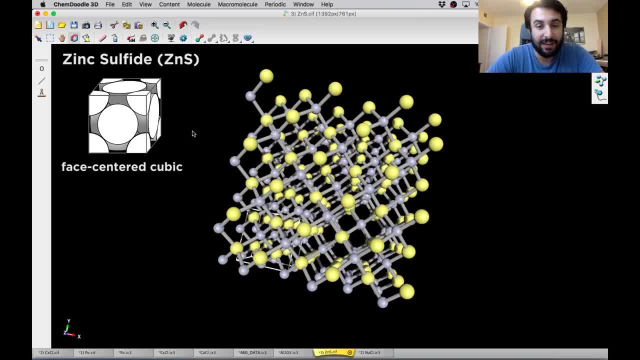 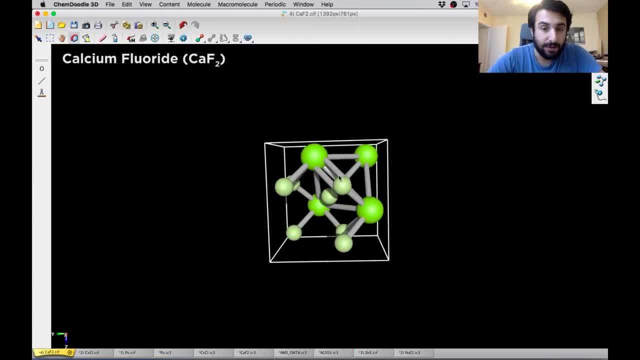 with the cation filling in the gaps, And we can see the reverse as well. So let's take a look at something else. So now we're looking at calcium fluoride, So we've got Ca2 plus ions in green And then the F minus. 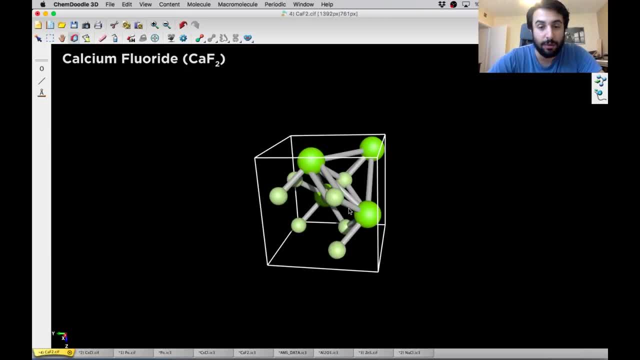 fluoride ions over here. These are the smaller ones, And so now we're looking at something where we've got a one to two ratio. Earlier we were looking at one to one ratios of cation to anion. Now we have one calcium ion for every two fluoride ions, So we can see the discrepancy in the number there. 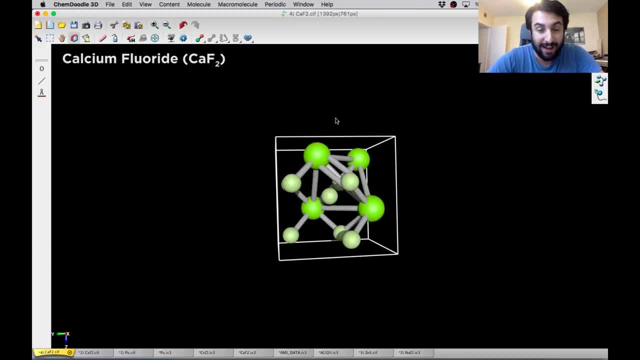 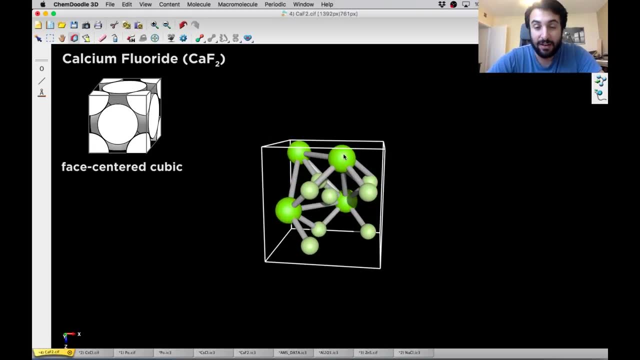 And now we're also looking at again. we're looking at a difference in the size of the ions. So it is actually the calcium ions, the cations this time, that are going to form the face centric cubic structure, while the fluoride ions are going to fill in the tetrahedral holes, Though in this case, 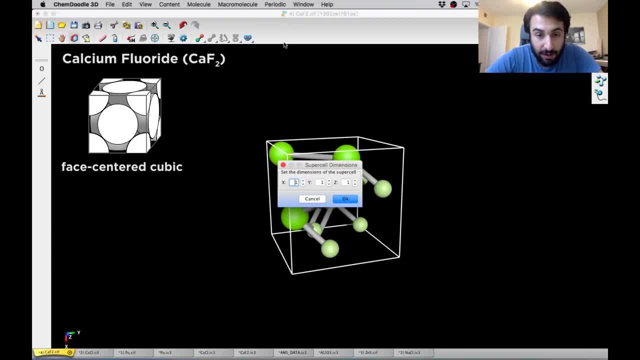 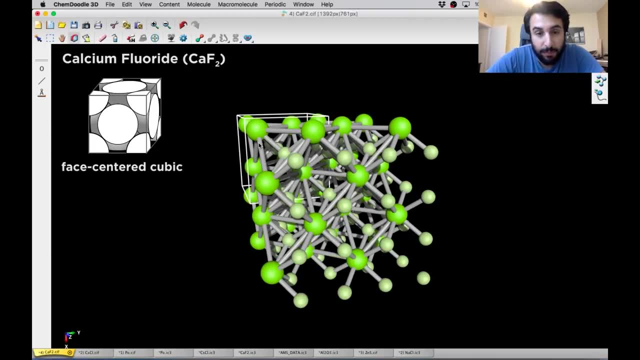 they will only fill half of the tetrahedral holes. So let's go ahead and build this out just a little bit. 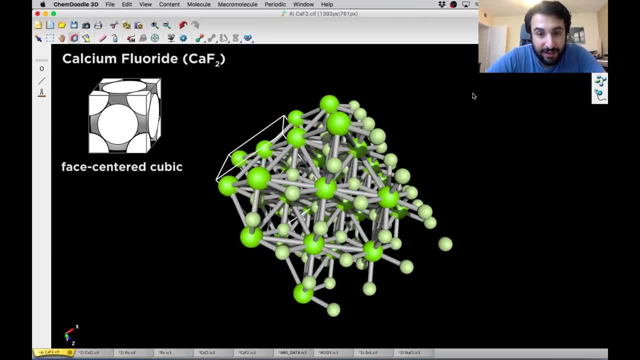 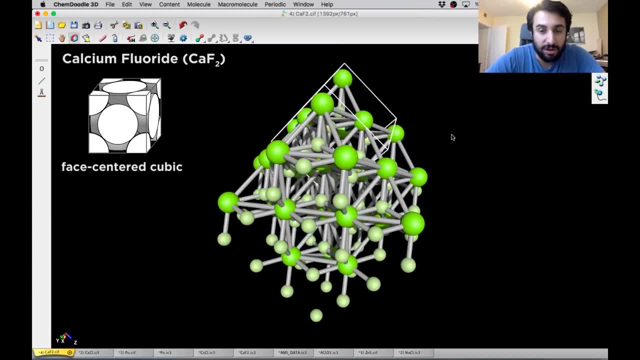 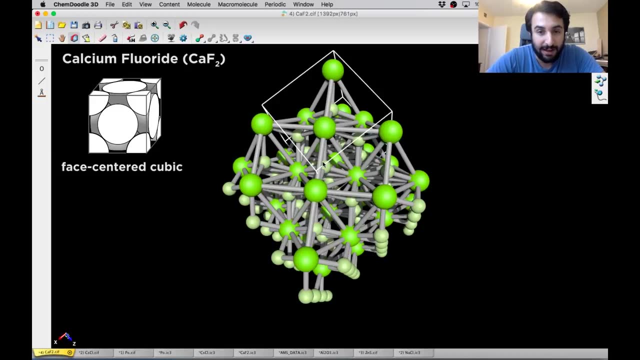 get a better sense of this, And so this is obviously a more complex unit cell because we're not one-to-one, right. This is not as simple as cesium chloride, where we can just have repeating cubes. right, We do have to allow for the fluoride ions all to be making contact with. 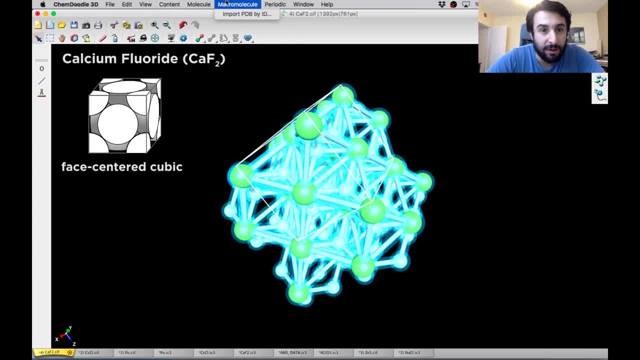 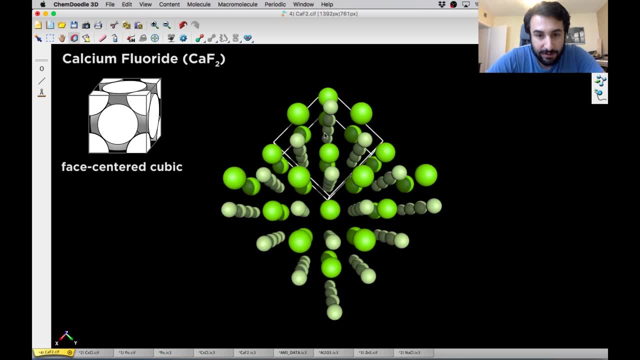 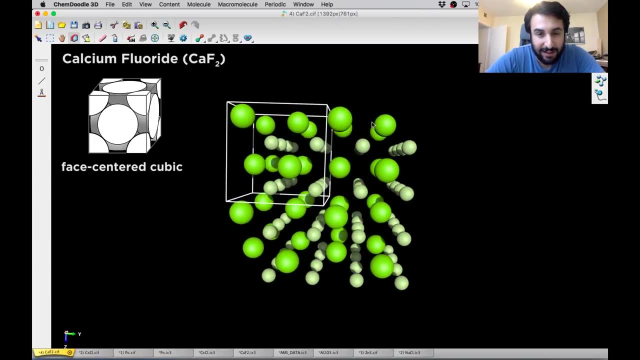 these calcium ions And we can get rid of these bonds. Sometimes it's easier to just remove the bonds so we can get a better sense of how this looks. So that's this one, a little bit more complex, And once again, we saw previously that the anions were forming the face-centered cubic. 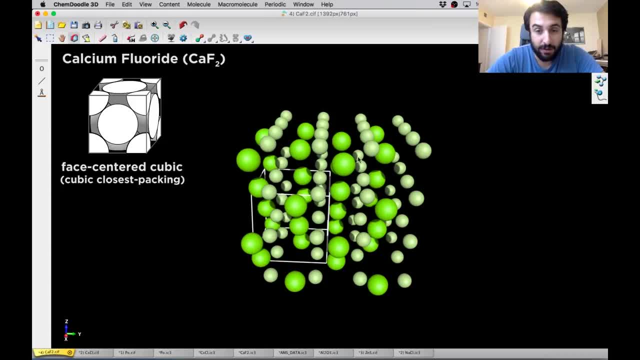 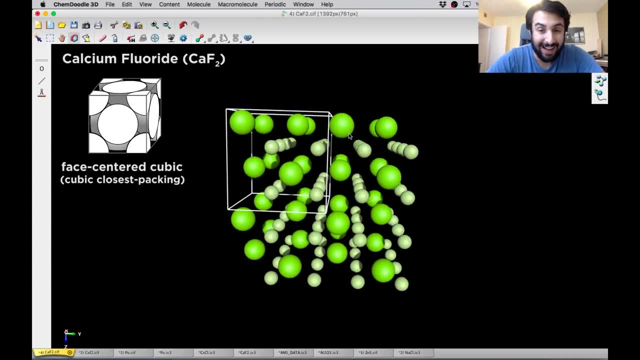 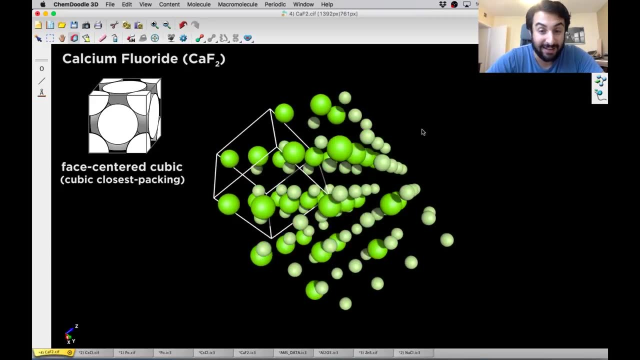 also known as cubic closest packing- So that's another way of calling it- with the face-centered cubic structure. So earlier we saw the anions forming that structure, Now we're seeing the cations forming that structure. So once again, it just depends on the relative sizes of the ions in terms of what these are. 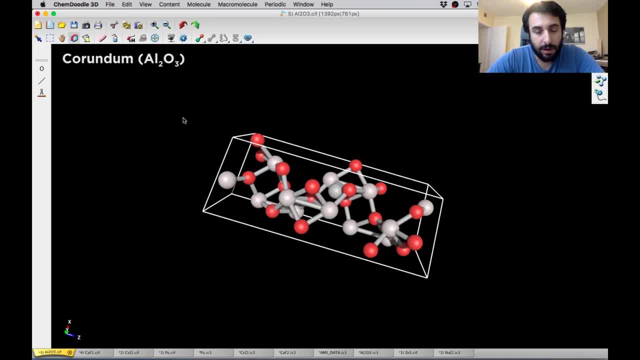 going to do. Let's go ahead and look at one more. So here we have a form of aluminum oxide called corundum, So this is Al2O3.. So it's even more complex in terms of the ratio between the cation. 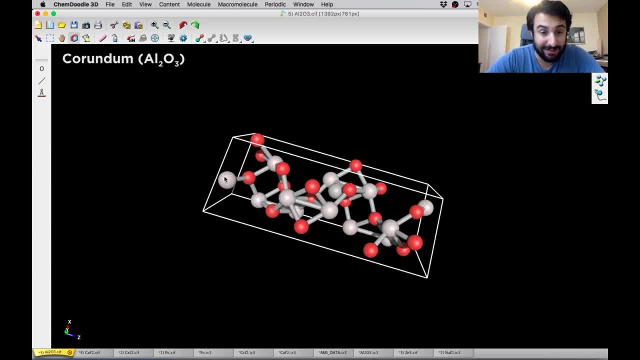 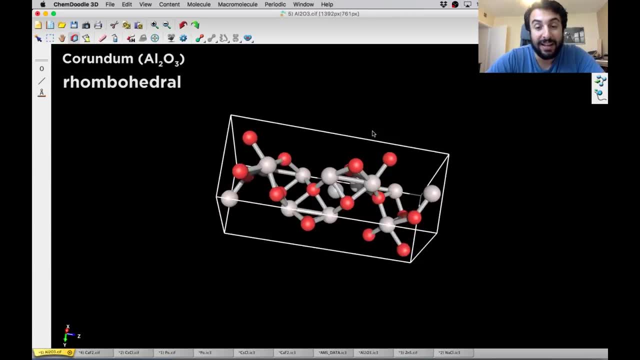 and anion. So we've got Al3 plus in gray and then O2 minus in red And this is going to form a rhombohydrate. So this is a rhombohedral structure. So they're not all cubic And there's actually many, many of. 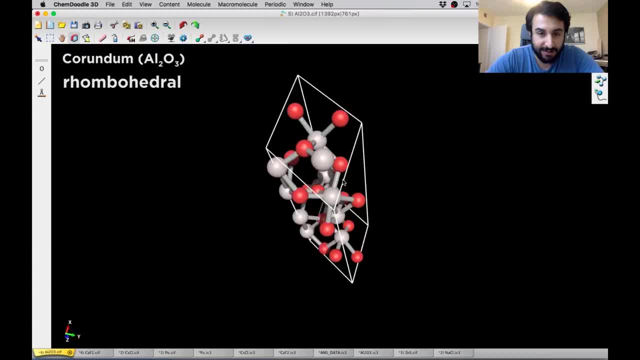 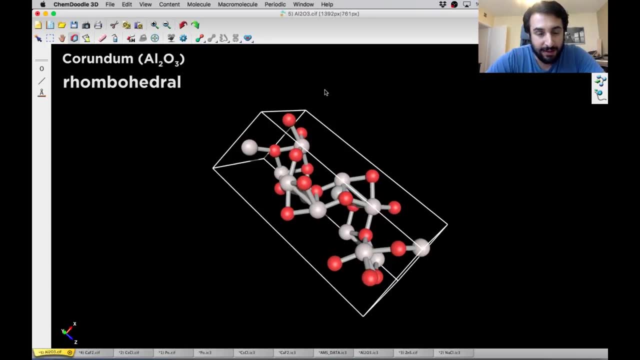 these, So we won't go through all of them, but I wanted to show you one weird one, And so this is called rhombohedral. We can see that it's not at all like the cubic structure that we looked at, And so let's build this out once again, just a little bit. Let's just do three of these, since 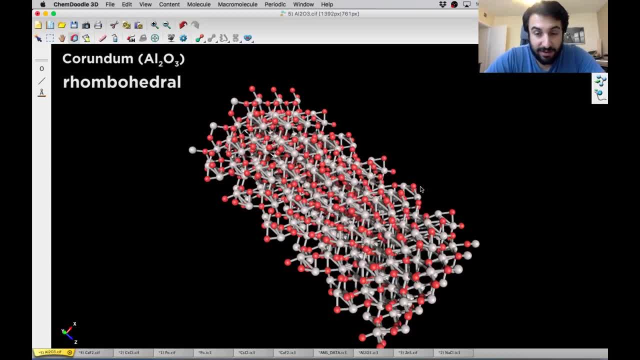 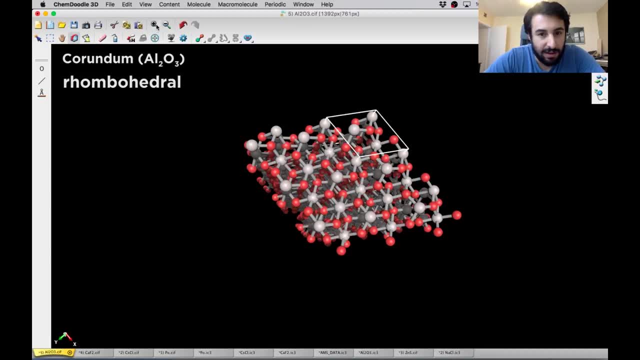 it's rather complex. So here's that. We've built the unit cell out quite a bit and we can look at this from a few different vantage points. We can zoom in if we like and really get a good look at this thing. We can also once again get rid of.